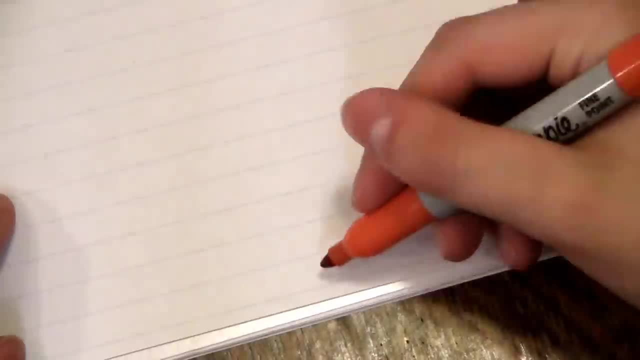 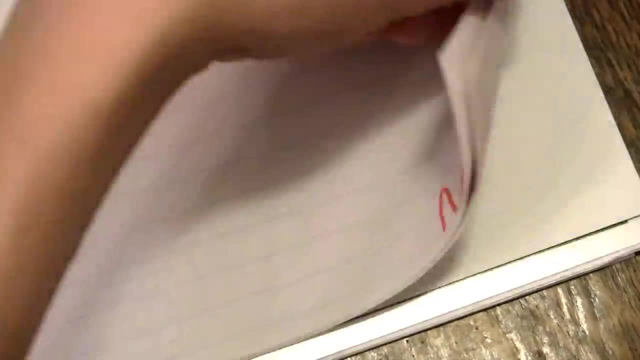 or add another dot in the next place in the spiral, or how about keep making the squiggles squigglier? But what does squigglier really mean? Like you could just increase the curvature of the squiggle, or you could make it squiggle more between the squiggles. You want to figure out an. 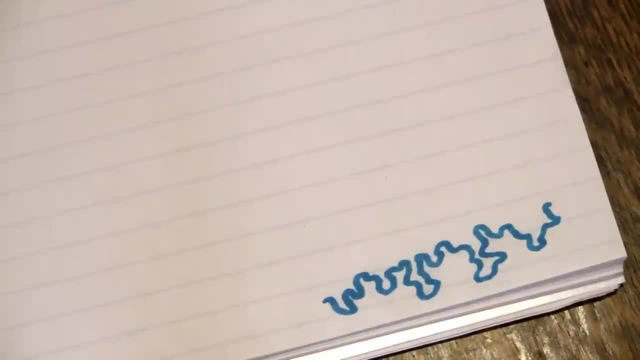 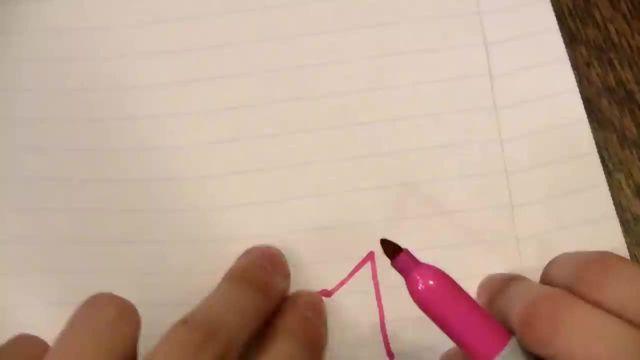 exact squiggle rule so that you can really get into the squiggle zone. so you discretize the squiggle into a zigzag line and you can make it squiggle more between the squiggles. On the next layer you could just deepen the zag or you could put a new zigzag on each old zig and 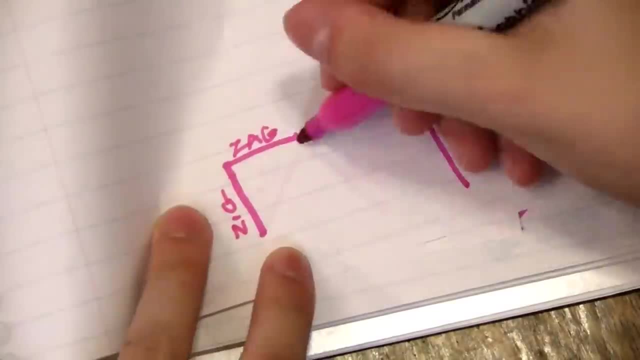 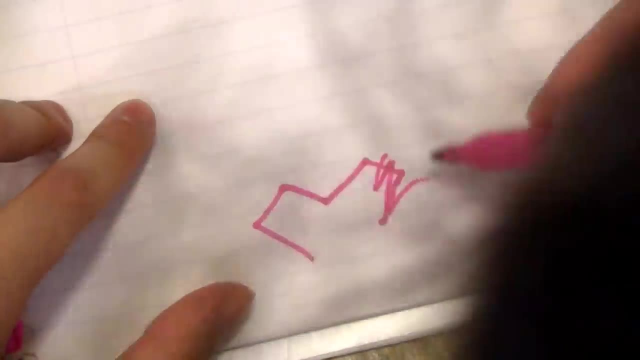 zag. Or maybe zigs should get a zigzag and zags should get a zagzig. So the next would be zigzag, zagzig, zigzag. wait, no, that was a zag, and those get turned into zagzigs, so it should be. 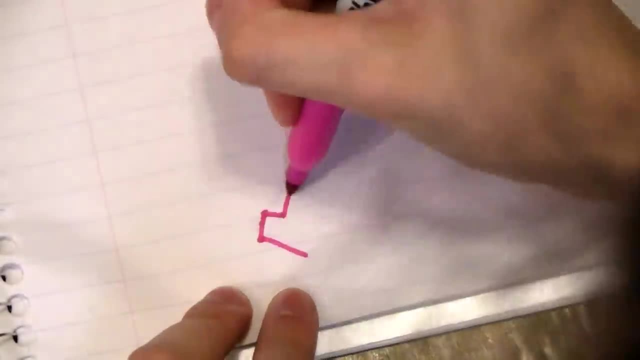 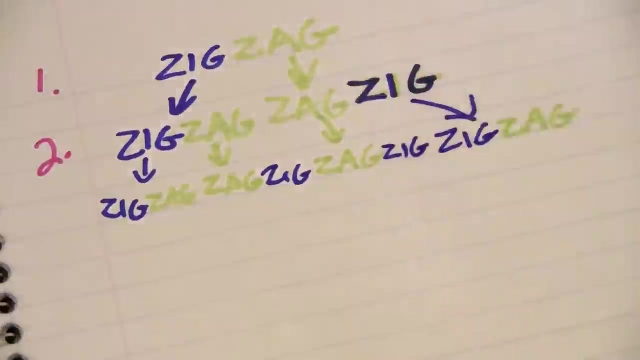 zigzagzagzigzagzigzag And next zigzagzagzigzagzigzagzagzigzag. wait, was this a zig? Maybe if we put it all into some sort of reference diagram that generates each new pattern based on- no, this was supposed to be about mindless zigging in the squiggle zone. This 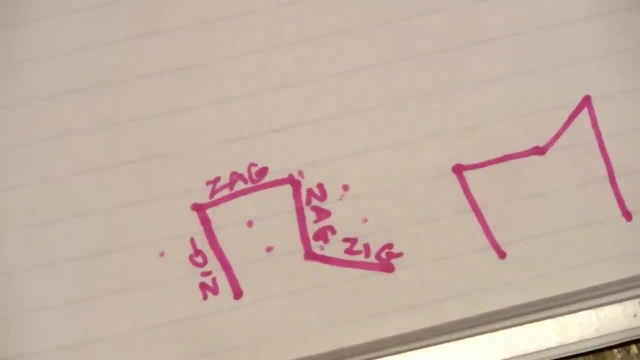 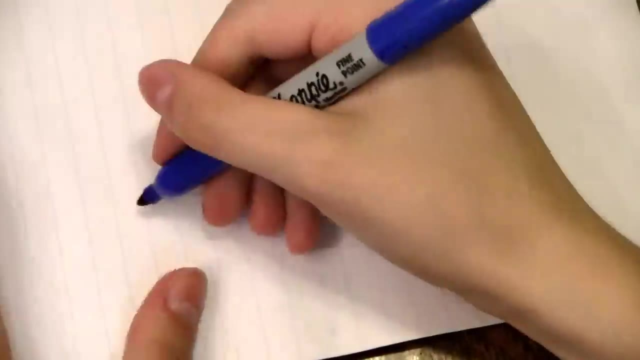 is unacceptable. So maybe just pretend each time you get to a new stage, the old path is all just zigzagzigzagzigzagzigzag. And to keep it all neat and orderly, you decide to try to make all the lines the same length, always with right angles between them. Here we go. 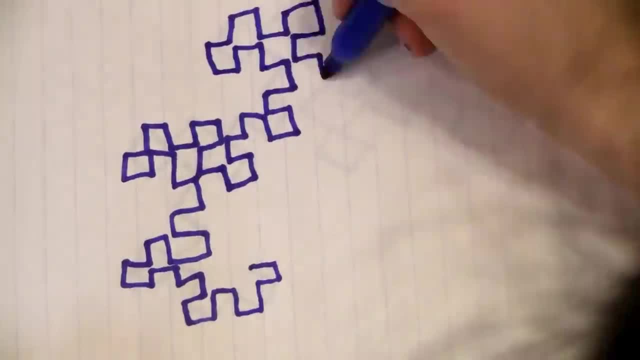 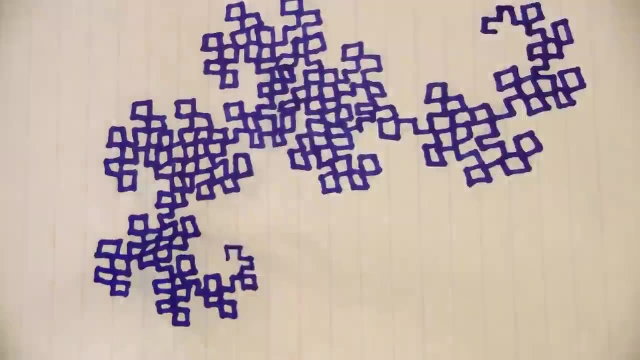 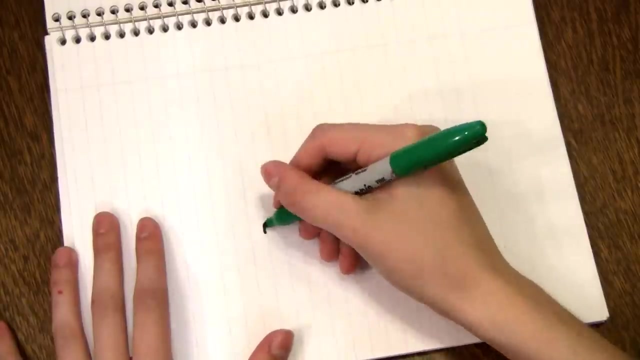 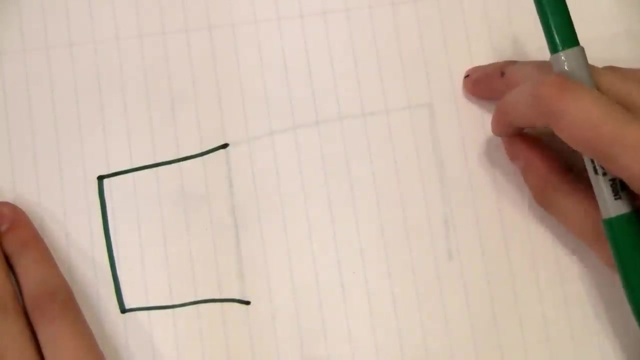 Wait, how did this? uh huh, what if you tried starting with three lines: Zigzagzug. Okay, so then each zig should get a zigzagzug, and each zag a uh zagzagzig, and then the zug gets. 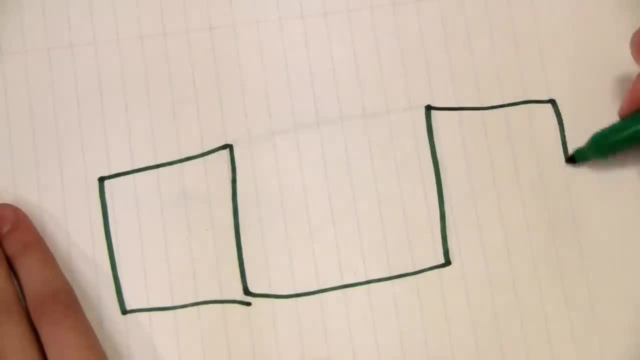 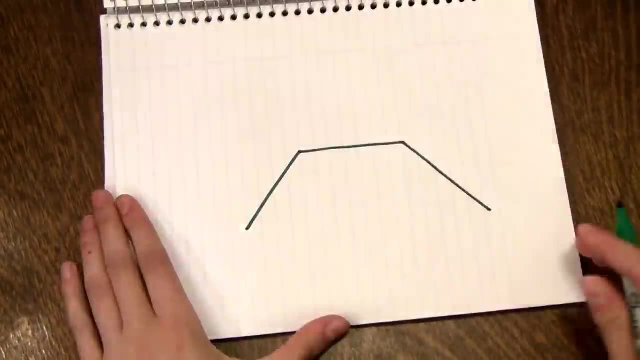 well, maybe it just goes back and forth, whether it's goes on the inside or the outside. okay, wait now, where did it start? and everything's running into itself and it's getting bigger and doesn't fit on the paper. okay, maybe if it were a little more. 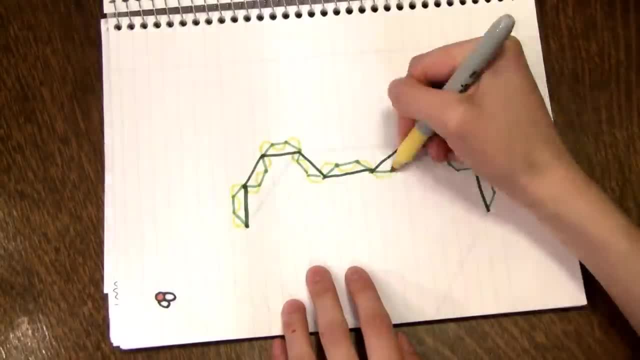 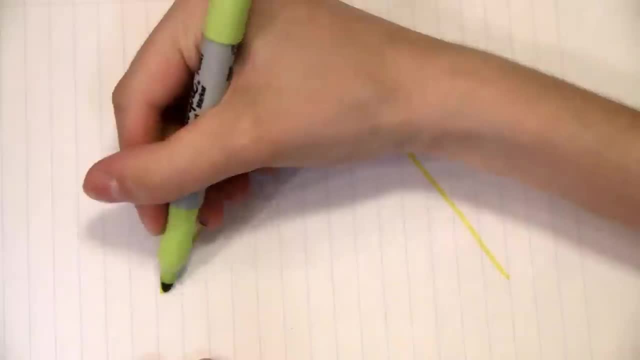 open, it wouldn't run into itself. say, like half a hexagon so you can keep all the angles perfect and then trapezoids in and out. yeah, this is totally gonna work. look at, in fact, like this you could even make it go inside first and back and forth and it wouldn't run into itself. 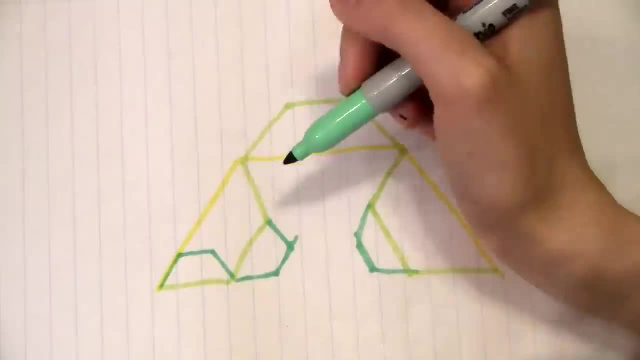 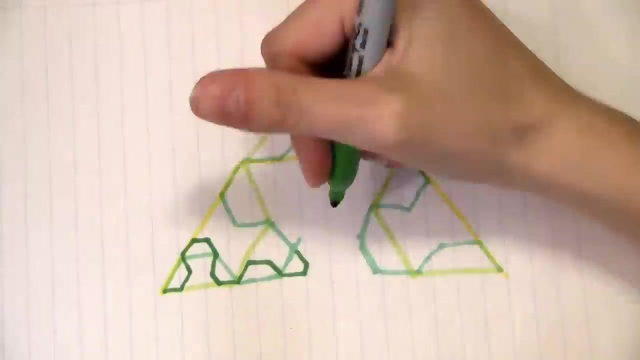 and next you could make it go even closer together here and still not run into itself. except that means you'd have to start on the outside this time. but that's okay, because next time you can go on the inside again. and now it's an easy pattern: trapezoid in, trapezoid out, trapezoid in. 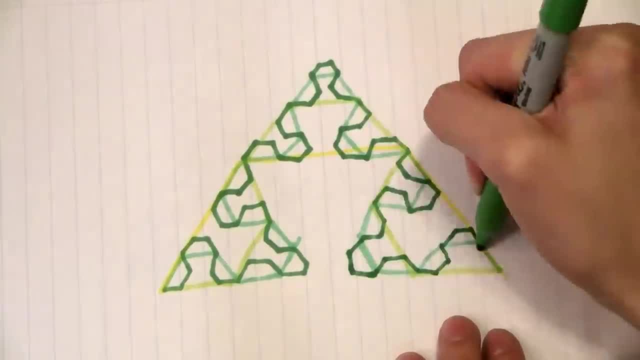 trapezoid out, back and forth until it's the last trapezoid in and then the next time starts with trapezoid out, although it's hard to tell what's in and what's out now that it's getting so squiggly. 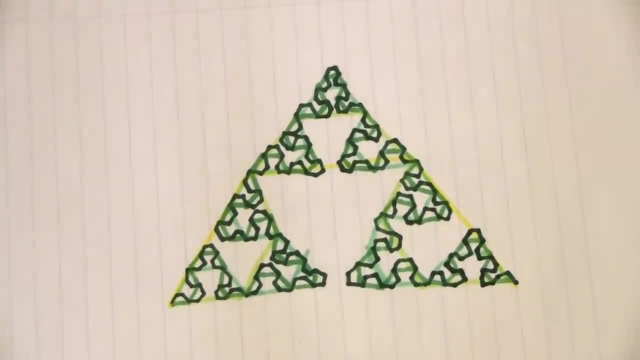 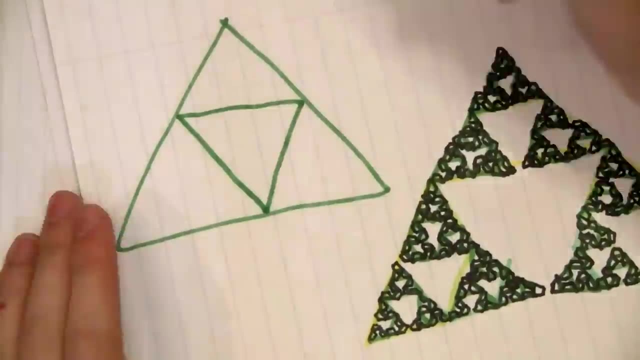 so you're just focusing on going on one side of the line and then the other and wait. this looks familiar. is that sarpinski's triangle? the fractal you get when you put a triangle inside a triangle and then triangles inside the new triangles you made, and then triangles inside. 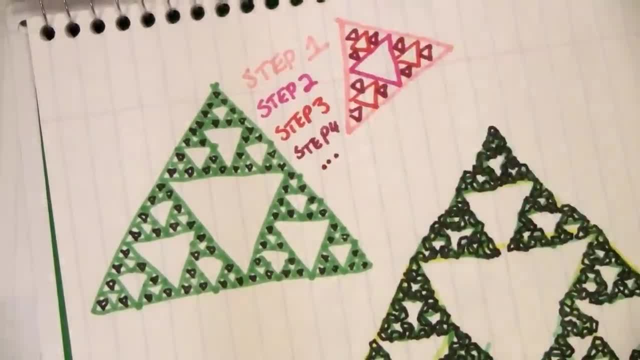 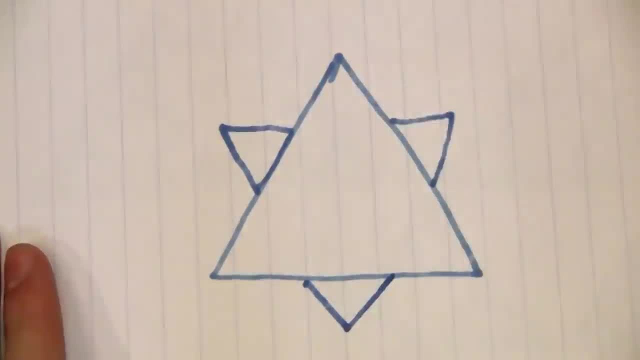 those new triangles? and why would filling triangles in with triangles give you the same thing as a trapezoidal meta-squiggle? Or is it the same thing, Which reminds you of another fact- all made of triangles, where you make this snowflake by adding triangles to triangles? 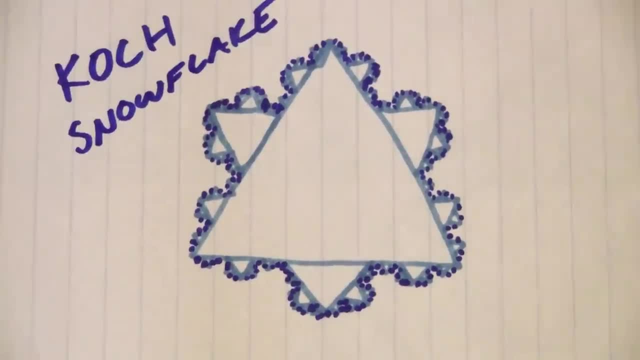 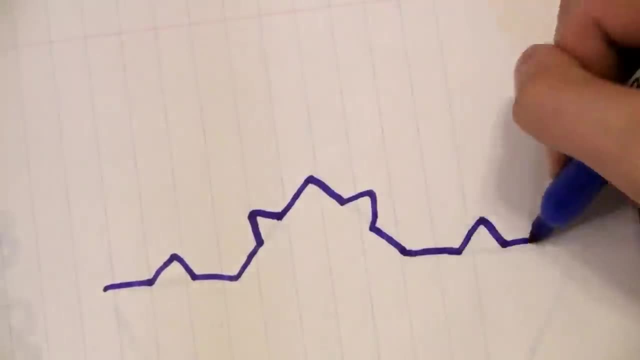 each one in the middle. third, of each piece of edge which you realize you could totally get with your tracing method: Start with one line with a bump, then trace each line to be a line with a bump, and so on, which is interesting because this time you're not squiggling back. 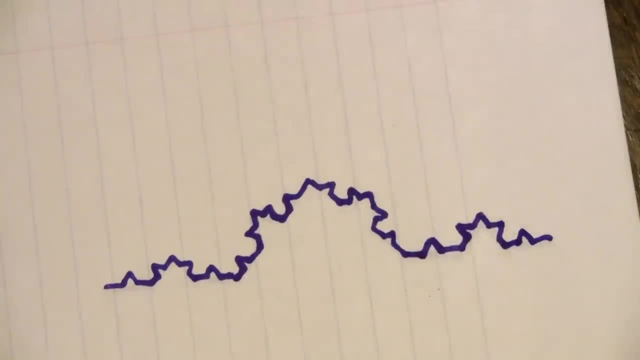 and forth, or forth and back, but bumping out the same way each time, though you could try doing it the other way, which makes you really want to know what you get if you do the first thing, but instead of always starting by zigging out, you alternate starting zig out and zig in. 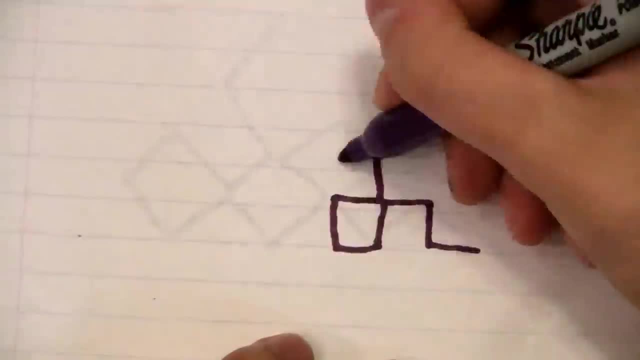 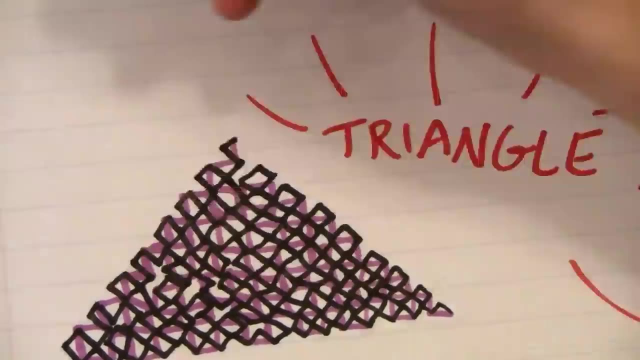 and it's kind of bumping into itself, and this would definitely be more perfect with graph paper or something. okay, now it's starting to look like a triangle- On the one hand, not nearly as cool as the spirally thing you made, but on the other hand, it's kind of like a triangle and it's 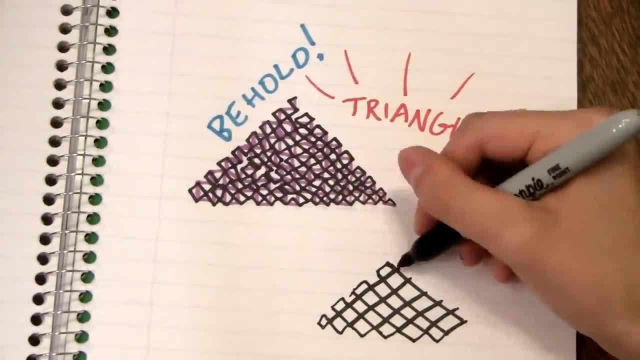 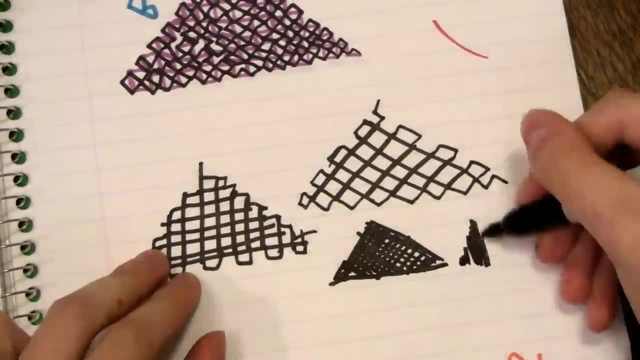 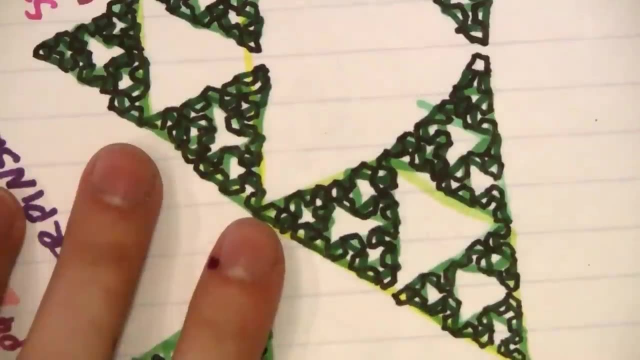 like a solid triangle too. If you kept doing this forever, would the triangle just fill up completely? These didn't do that, although with this thing, you have sections that are starting to fill up. Maybe here at some point that will happen, though it seems like it's just full of. 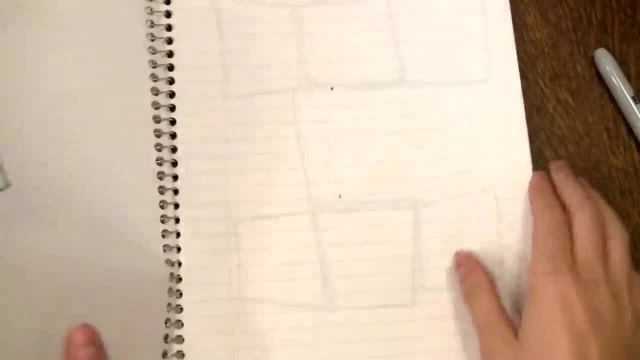 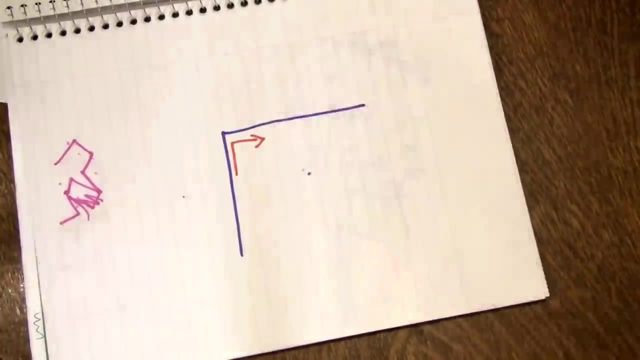 holes forever. You kind of wish you had a way to take some graph paper and skip all the way to what happens later in the sequence. Maybe if you had some sort of diagram like this: has a line with one right turn, the next one goes right right left, then the next goes right right left. 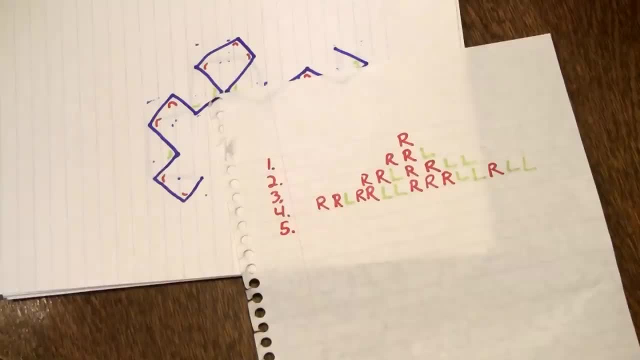 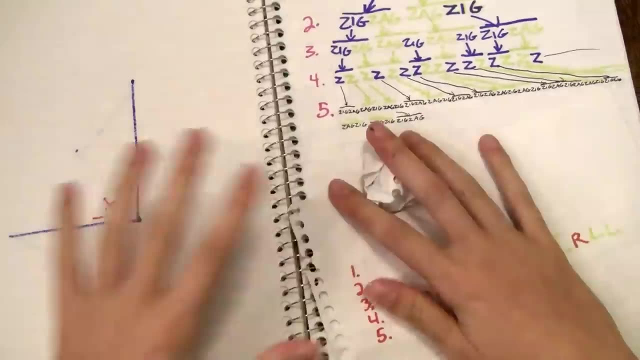 right, right, left, left. Is there a rule? Maybe it's just like the zig zag, zag zigs, or maybe not Okay, but there's probably some rule. Suddenly, a note lands on your desk from your friend Sam. 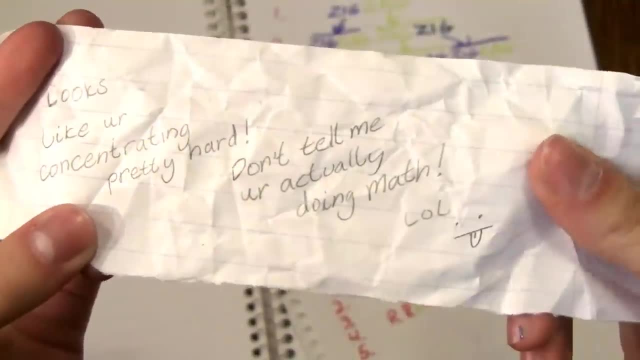 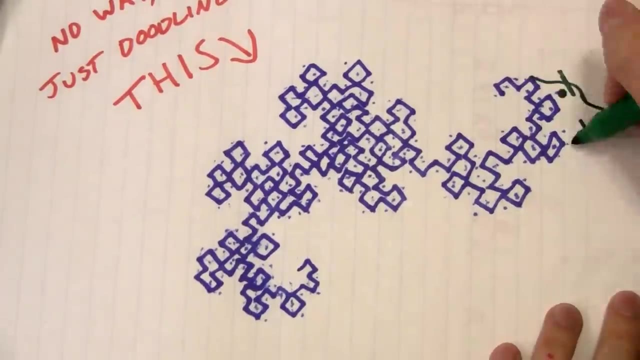 who writes looks like you're concentrating pretty hard. Don't tell me you're actually doing math, as if You write back. no way, I'm just doodling this and just to make extra clear: it's not math. You turn it into a dragon and name it the. 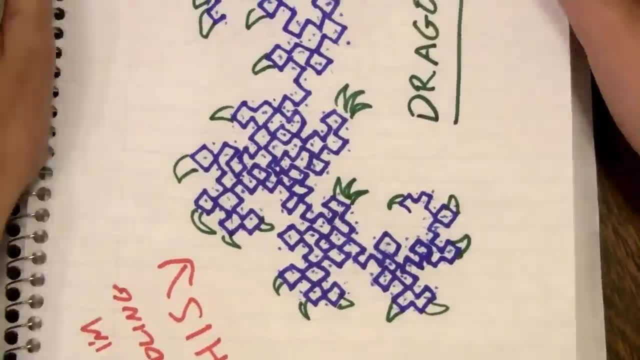 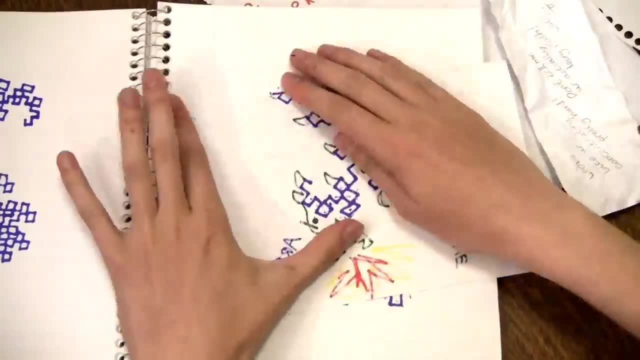 dragon curve. Yes, You don't want to crumple up your awesome dragon doodle, but you do have to throw it two rows over so you neatly fold it into a note spear, which just means you're folding it in half again and again until it's easy to javelin across the room, the moment the teacher's back is. 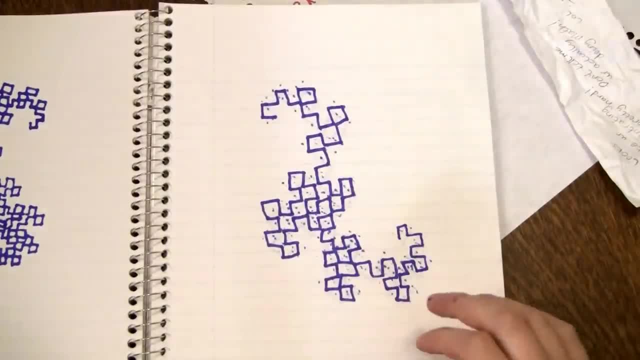 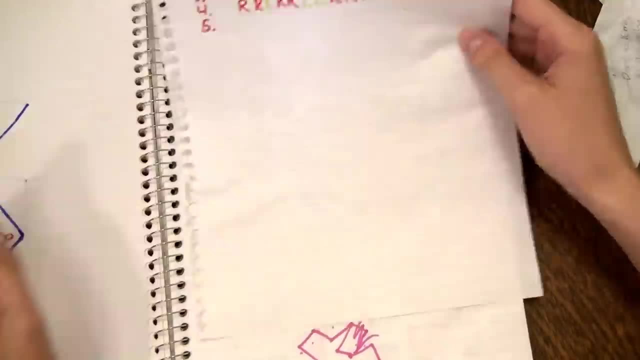 turned. Bam yes, perfect landing. You watch as Sam unfolds it and suddenly you feel like you see something familiar, some sort of similarity between the paper. and is that possible? You take your diagram and fold it in half and in half again. You see that the paper is folded in half. 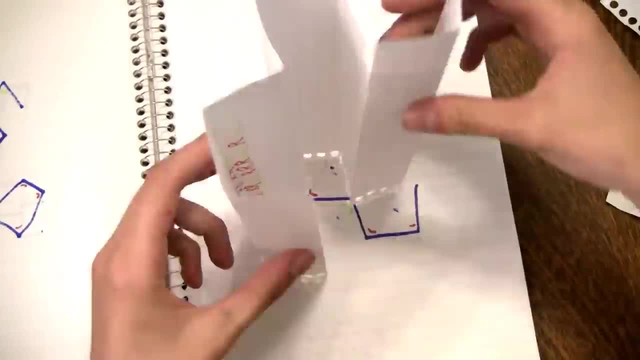 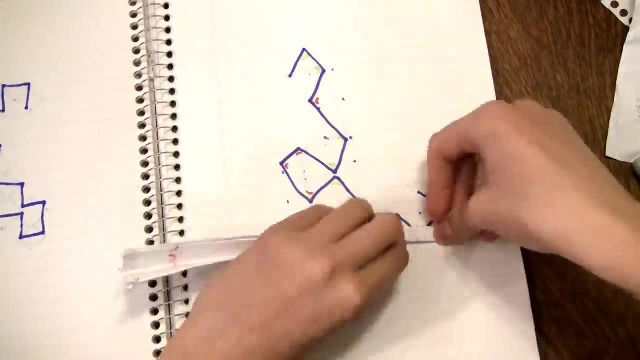 again and again, And wow, not only does it look like it's doing the same thing, probably, but it's also showing a new way to do it. Instead of keeping track of zigs and zags, you can just copy the old. 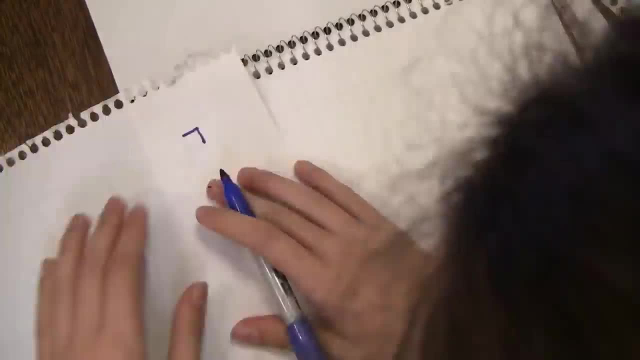 one and add it 90 degrees from the other, which is totally traceable, Bam, easy. Well, as long as you can keep track of what end to start from, And you don't even have to keep track of what order to draw. 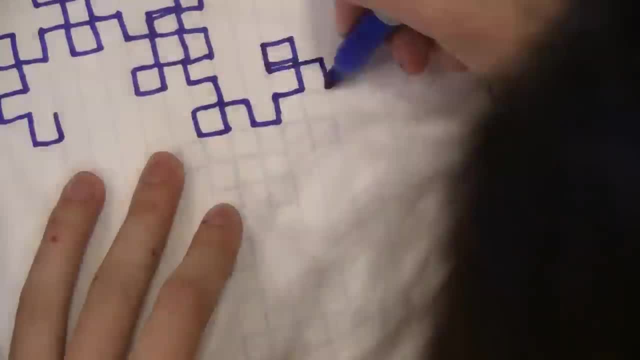 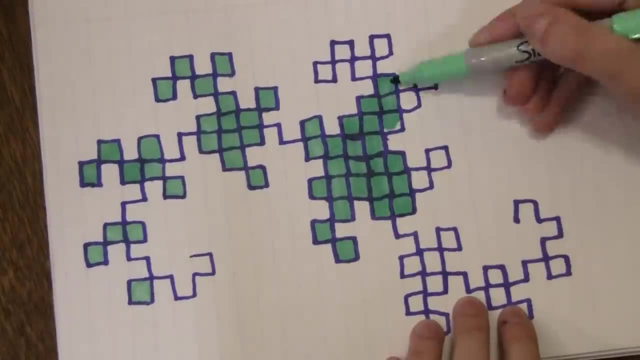 the lines in. you just need to keep things roughly on a square grid so things line up Easy, Until it gets too big for your paper And you have to dragonize it. It's funny because one way it gets bigger and bigger If you go on. 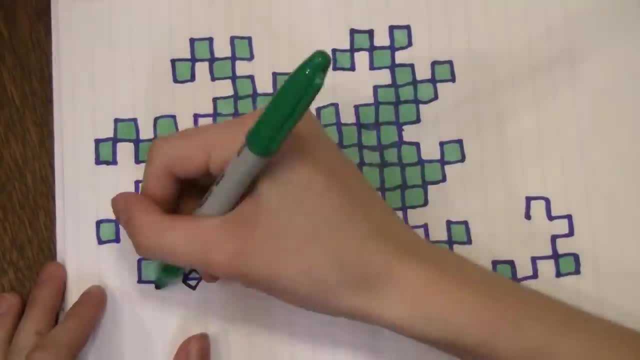 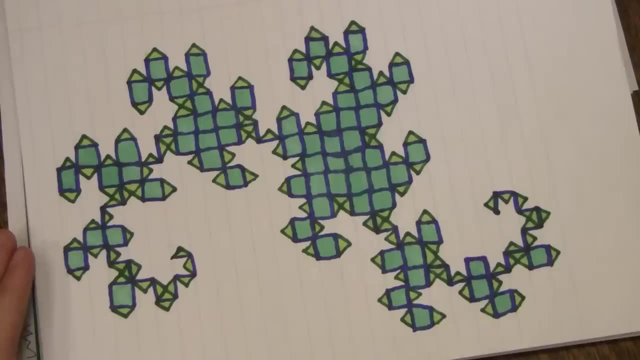 forever it'll be infinitely big, But with the first way it stays basically the same size. you just draw more details, Which means if you do it forever, the line will still get infinitely long, but the total size will stay the same. Would that even work, An infinitely long line all squiggled up into a 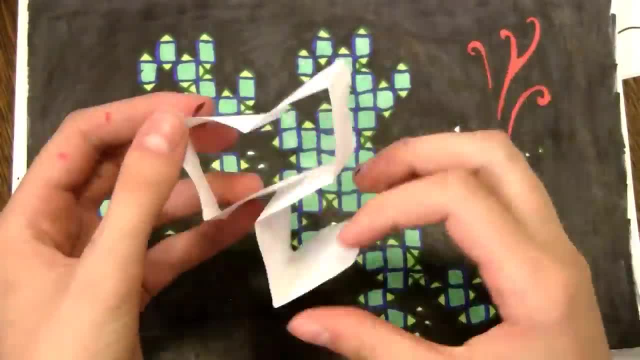 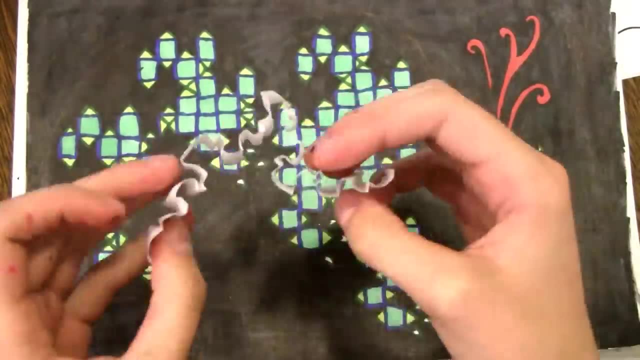 finite area, And then with folding paper, the whole thing gets smaller and smaller until maybe it disappears entirely, Which you suppose is the case. Maybe that would make sense, because the edge of the paper stays the same length no matter how you fold it.